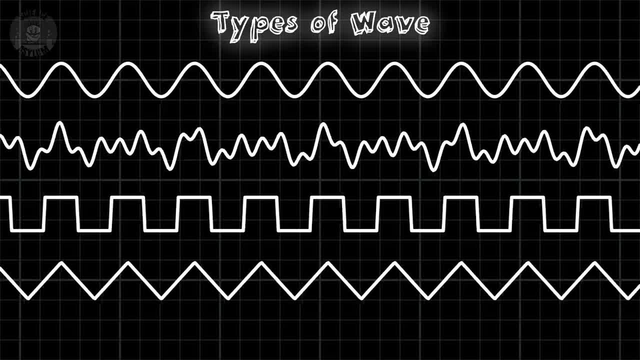 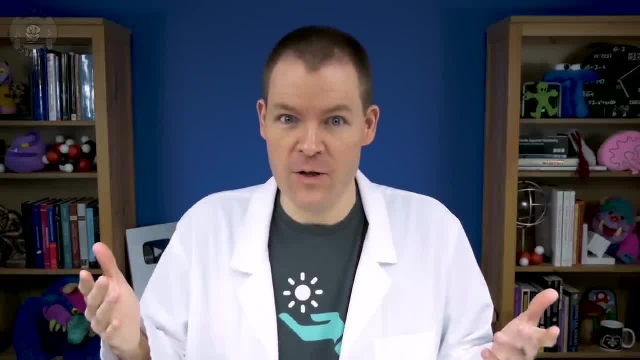 They could be irregular or boxy or even triangular. They just need to have that back and forth shape. So, yes, while wave is a verb, it's also a noun. Waves are things. Get on board people. Last but certainly not least, function. 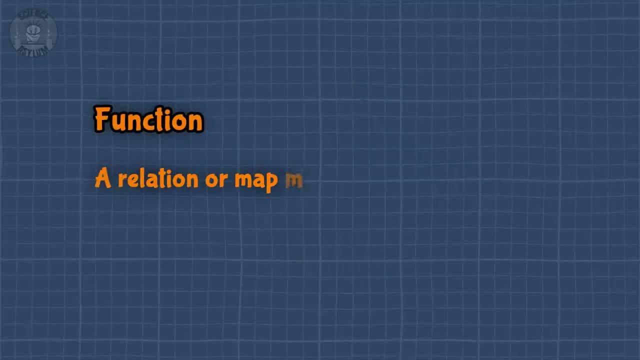 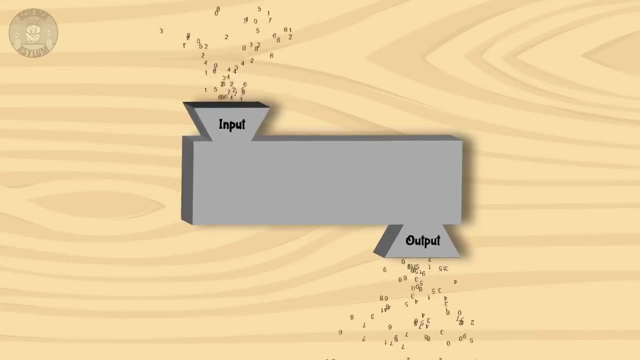 By that we mean a mathematical function Which is a relation or map between sets of numbers, But that's a bit abstract. It's easier to think of a function like a little mathematical machine. You put numbers in, like maybe time or something, and you get numbers out that depend on that. 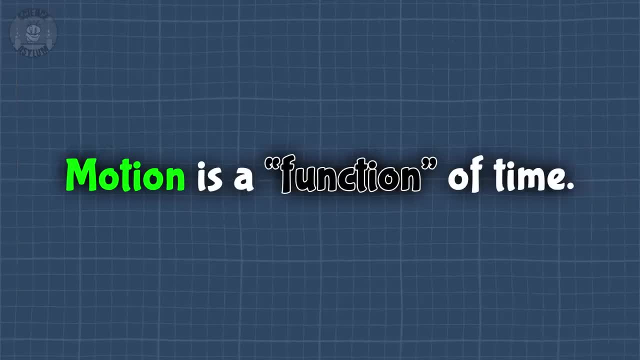 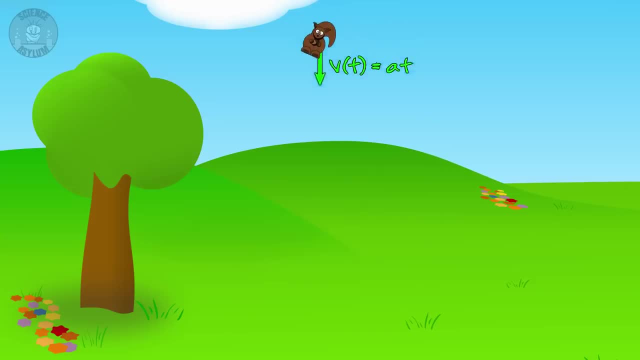 input Like the motion of a squirrel. We'd say that motion is a function of time, or just v of t for short. So this function tells you how fast a squirrel is falling at any given moment. It's just a way of showing that some measurements are accurate. 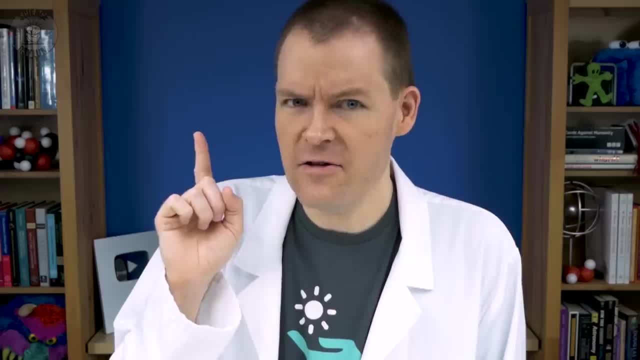 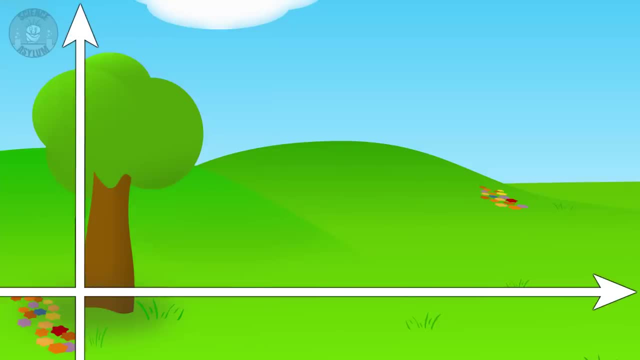 It's just a way of showing that some measurements are accurate And some measurements depend on other measurements. Now let's start combining words. A wave function is a function that looks wavy. Surprise, The falling squirrel function isn't wavy, though. 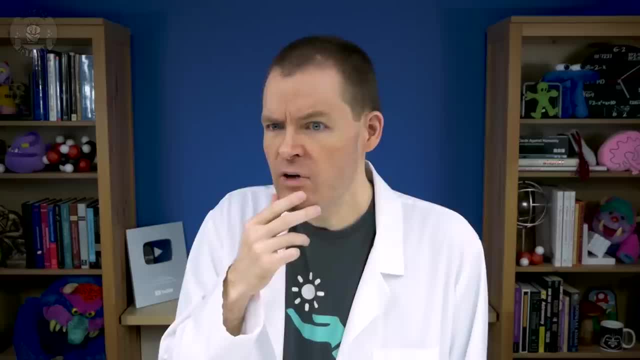 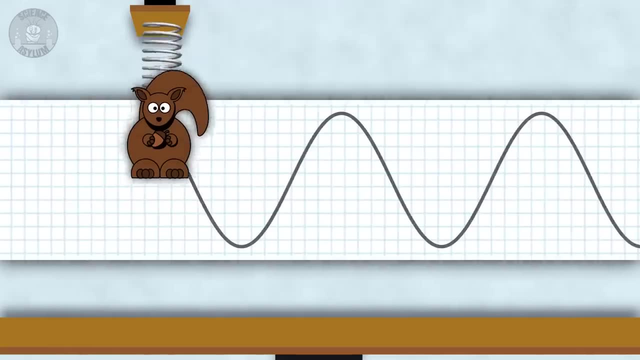 It's just a slanted line. There's no back and forth shape. We need a back and forth motion. Let's attach the squirrel to a spring and give it a little bounce, Put some moving graph paper behind it and bam, we've got a wave. 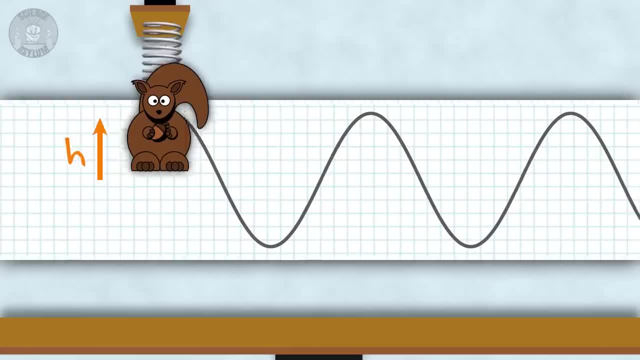 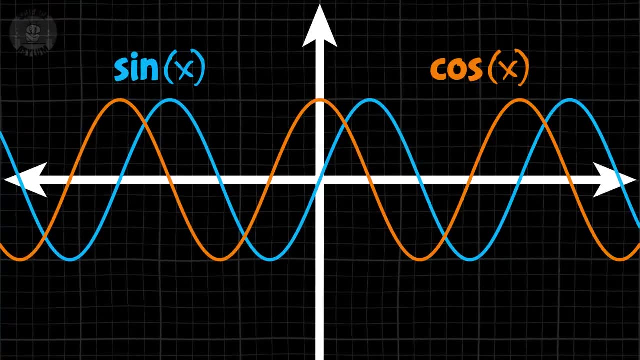 The height of the squirrel depends on time, so we say it's a function of time. Since its shape is wavy, we call it a wave function, And it's written using some kind of sine or cosine, because we know those look wavy. 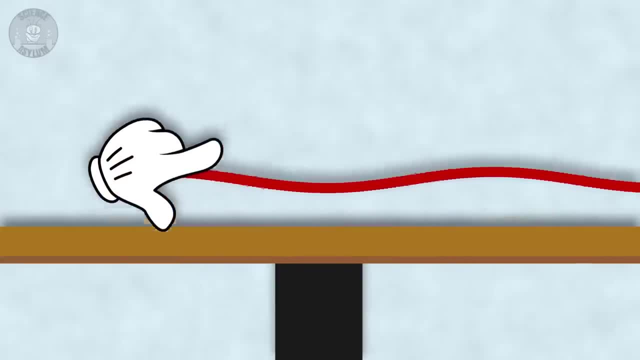 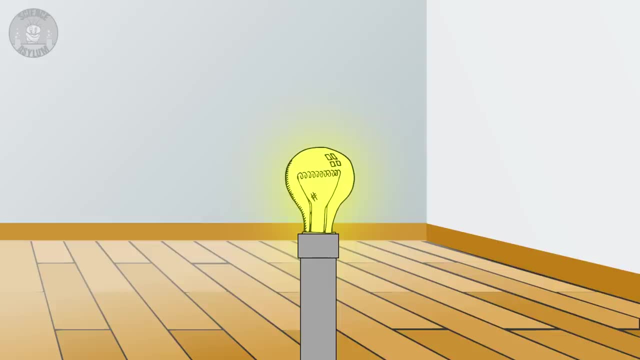 Bouncing squirrels aren't the only waves in nature, though. There are waves on strings. there's sound, water waves, AC voltage, waves on oscilloscope screens and even light, All of them involving some kind of sine or cosine. That's all there is to a wave function. 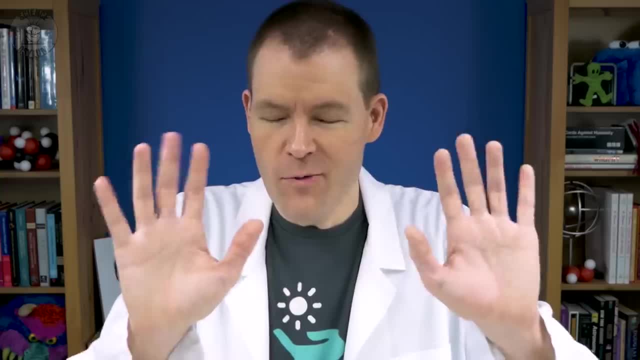 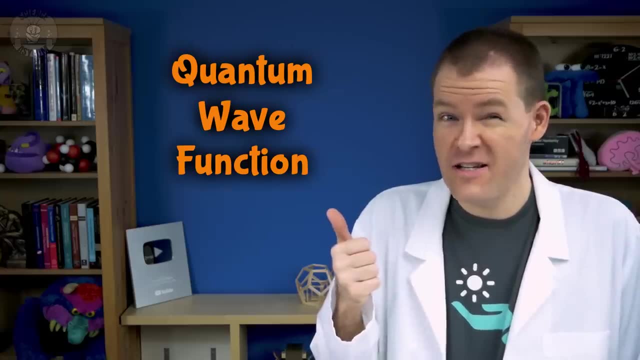 It's adding the word quantum on the front. that makes things weird, but we can handle it. Remember, we're not going to be doing this for a long time. Remember Quantum Brick Road. it's a journey. Ok, a quantum wave function is a wave function for quantum things. 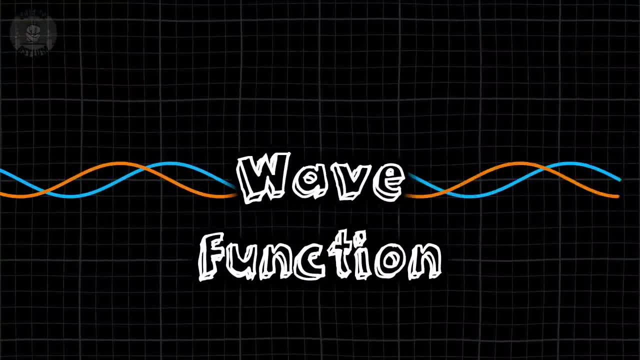 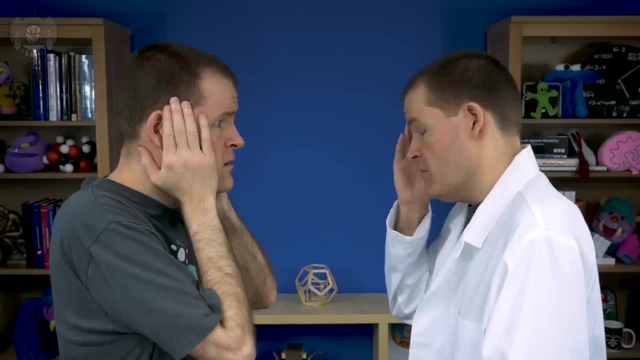 It shows a dependence between two measurements that has some kind of back and forth pattern and is about tiny particles. What two measurements? What's waving? What, what, what, Dude, calm down, Everything's going to be ok, Let's go deeper. 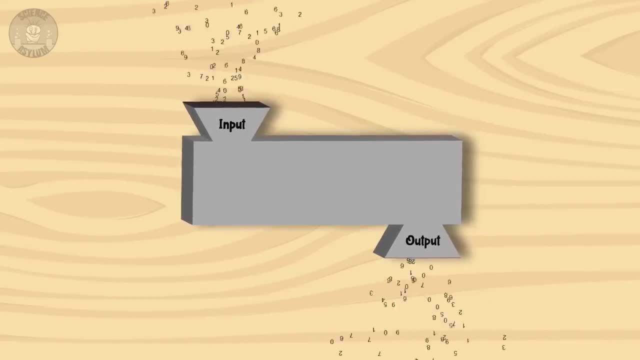 If a quantum wave function is like any function, then it's a little mathematical machine. You put numbers in and you get numbers out. The input is some measurable property about a particle, Where it might be what it might be doing when something might happen. 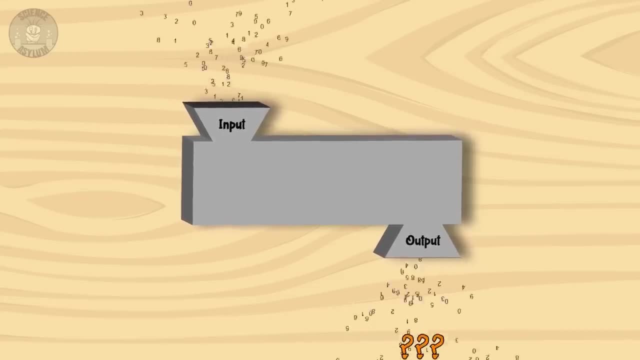 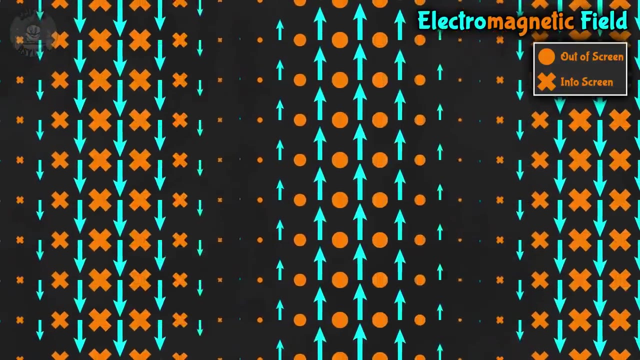 That sort of thing. The output- Well, that's the tricky part. See, with normal wave functions the output is pretty clear. It's some kind of distance or field strength or something else that's directly measurable. Quantum wave functions are a bit more abstract than that. 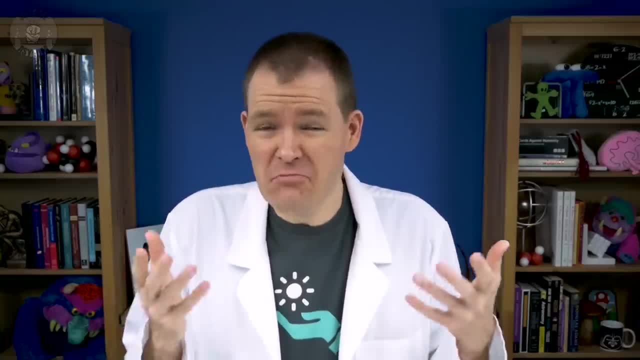 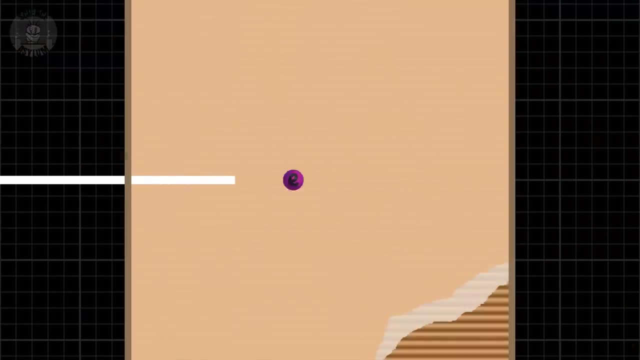 In fact, they're unobservable by definition. It might help to look at how they're used. I think it's time for an example. The simplest one I can think of is the particle in a box. For now, let's keep the box one-dimensional. 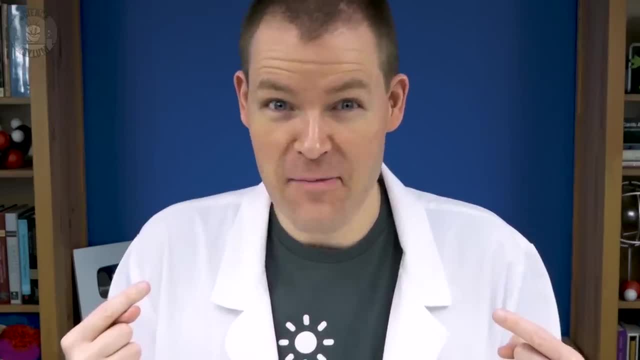 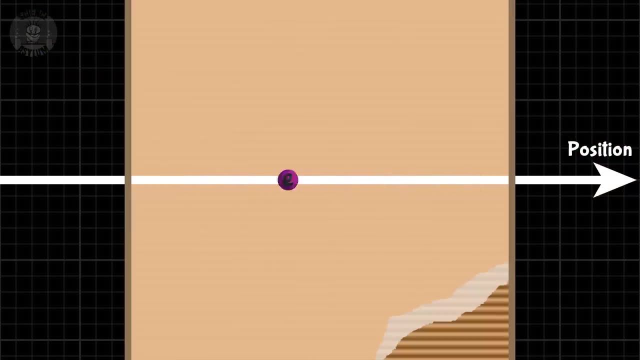 We don't want things to get too complex. Get it Complex, You'll get the joke later. Inside the box there's a single particle. Maybe it's an electron, but it doesn't matter, Just go with it, ok. 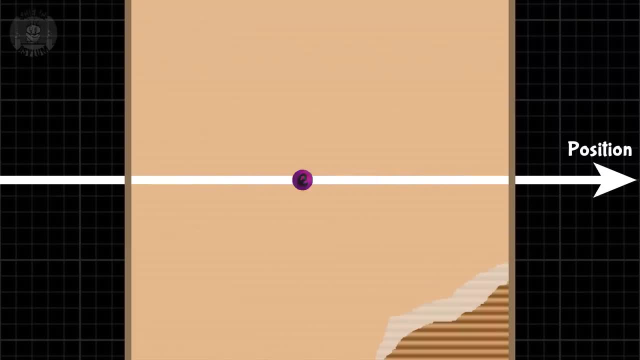 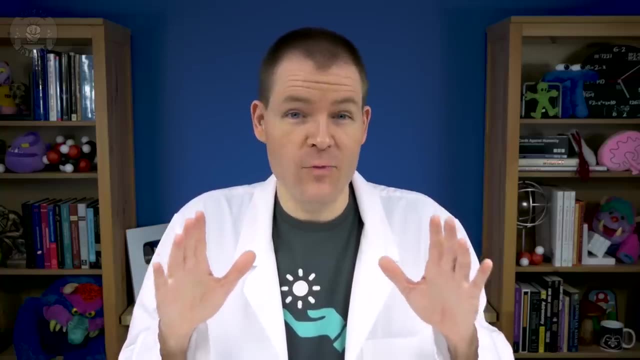 That particle has properties we might be interested in knowing something about. Where is it, What is it doing, And will it decay into other particles? Of course this is quantum mechanics, so we can't know anything exactly, but we can predict the probabilities of what those properties might be. 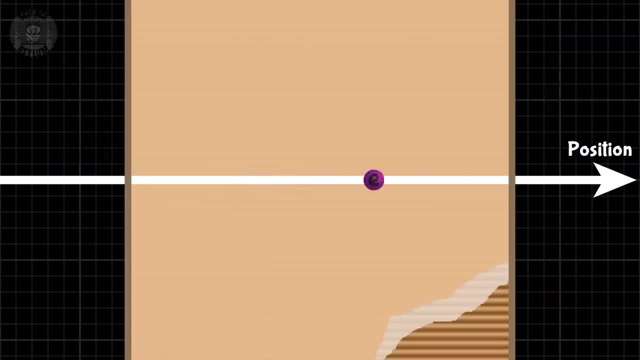 That's where the quantum wave function comes in. Say, we want to know where our particle might be inside the one-dimensional box. It could be just about anywhere, but it has a better chance of being in some places than others. Its quantum wave function gives us some idea of where. 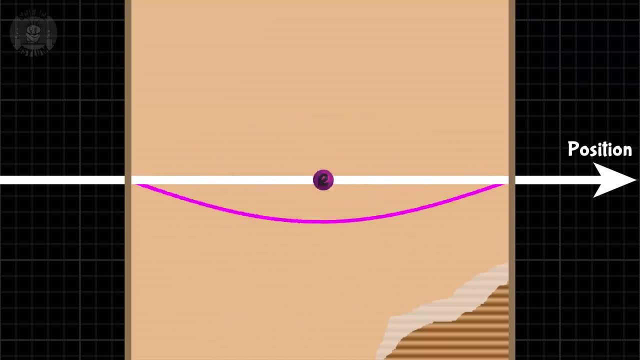 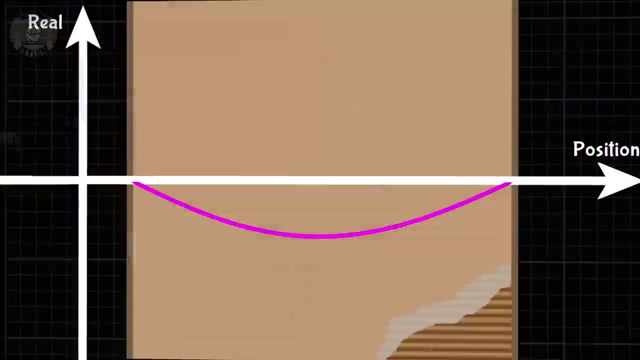 Just by looking at it, we can see that this particle has a better chance of being in the center of the box than on the edges. That's just a general idea, though It doesn't give us an actual probability To make matters worse. this isn't even really waving up and down. 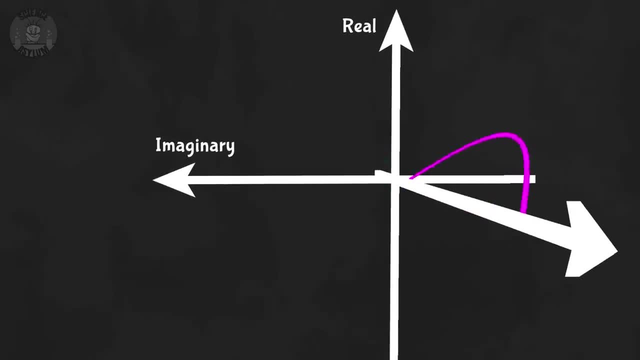 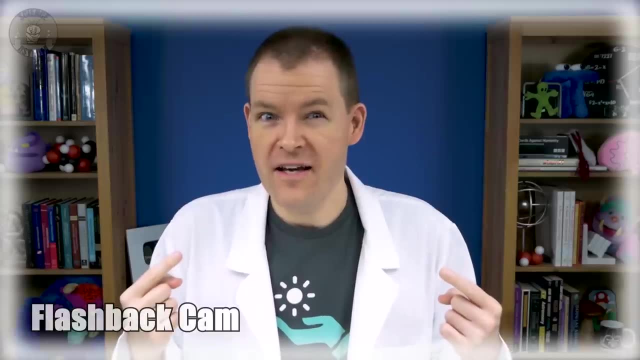 It's actually rotating through both real and imaginary numbers, the combination of which we call complex space. Hence that complex joke from earlier. We don't want things to get too complex. Get it Complex. I'm such a dork. The point is that the quantum wave function isn't even completely real. 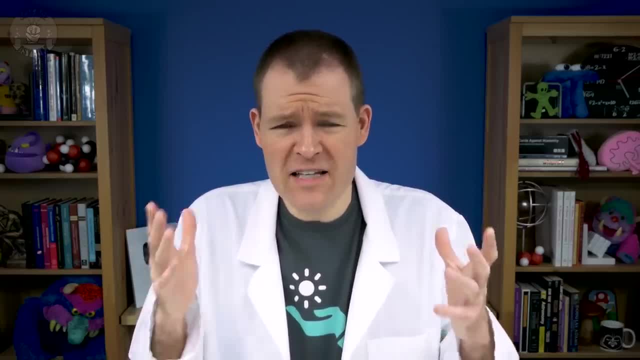 It's just a matter of how complex we want it to be. We don't want things to get too complex, We want things to get completely real, at least in the mathematical sense. But that doesn't mean we can't get something real out of it. 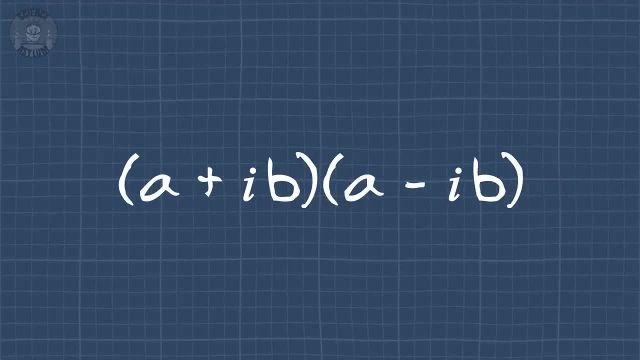 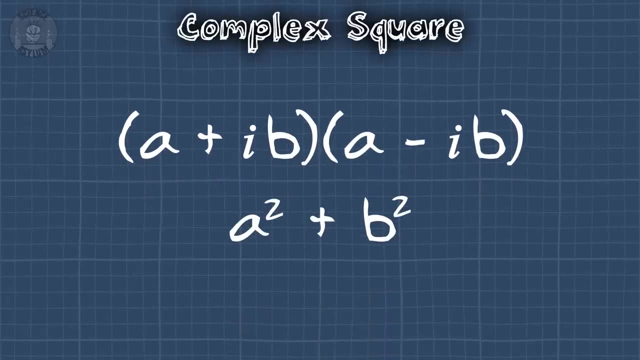 If you multiply a complex number by what we call its conjugate- that's just a sine swap of the imaginary part- then you've done something called a complex square. The imaginary parts cancel and you're left with only real parts. Just got real. 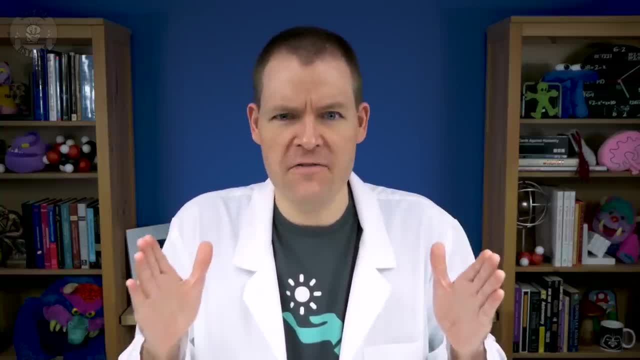 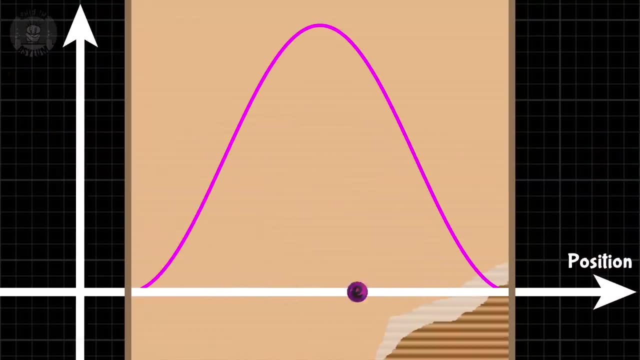 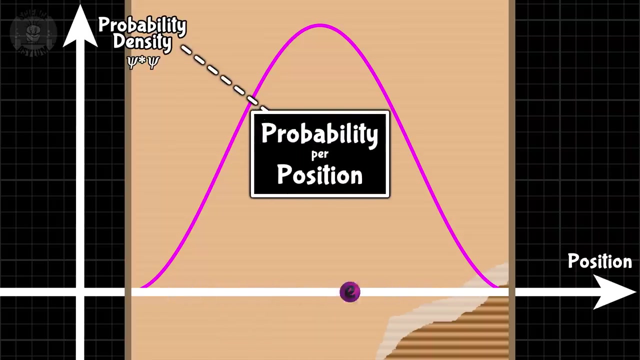 Jokes aside, now that we have only real parts, we can actually make physical sense of this. Instead of looking at the quantum wave function itself, we look at its complex square, something we call the probability density. In this case, it's a probability per unit length measured along our one-dimensional box. 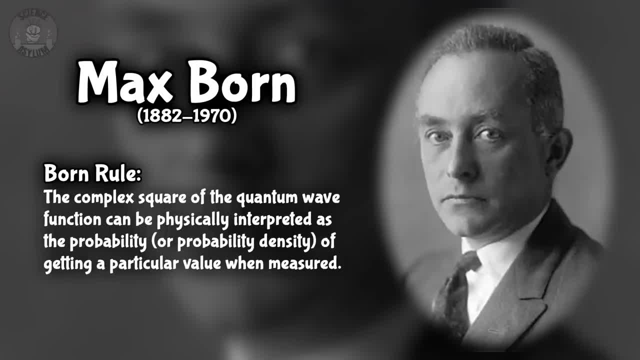 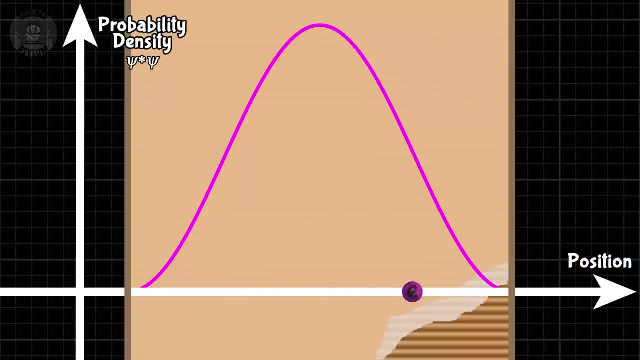 This view of the wave function is called the Born rule, named after Max Born, who came up with it in 1926. This realization was groundbreaking. So we'd say this is the probability density for position. It's best to think of it like a bunch of separate numbers along the box. 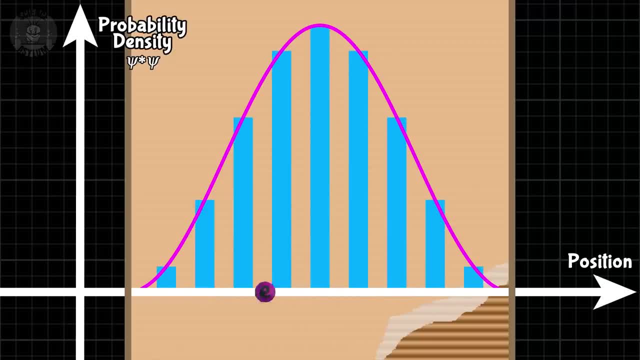 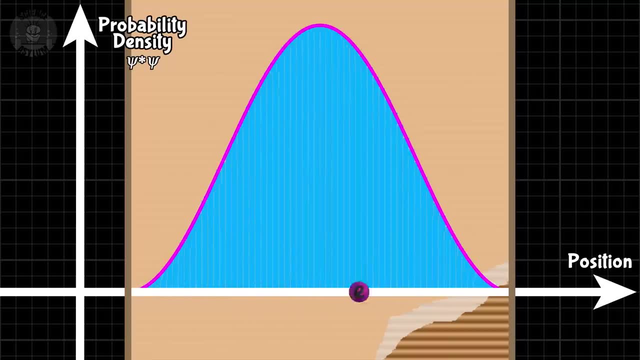 The height of each of these bars Is the probability density at that location. There are a lot of possible locations for this particle, though, so there are a lot of vertical bars, So many, in fact, that it all just looks like a shaded area. 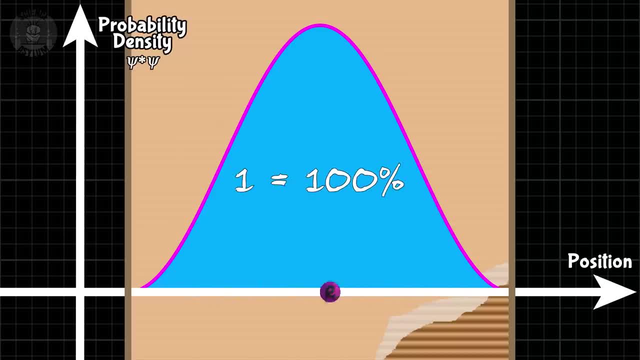 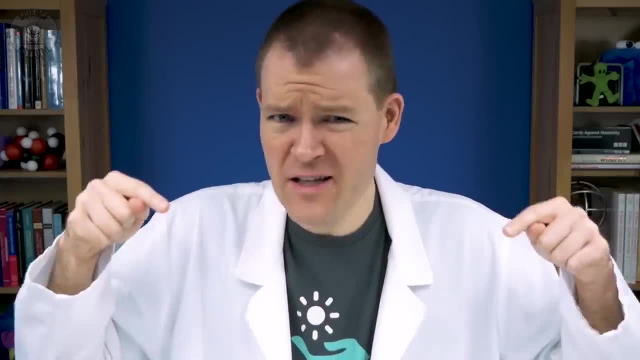 The total area covered by all the bars should be equal to one or 100%, Because there's a 100% chance of finding the particle somewhere in the box. I mean, we put it in there ourselves, right, But let's say we only want to know the probability of finding the particle between here and here. 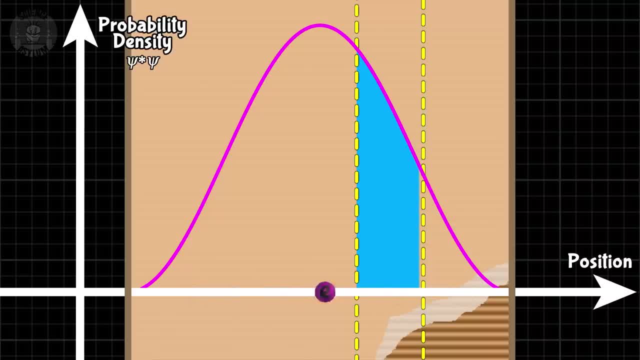 All we do is add up all the skinny rectangles between those two points And the shaded area is the probability. It's that easy. You can clearly see that some areas have a higher probability than others. What if I'm interested in something other than position? 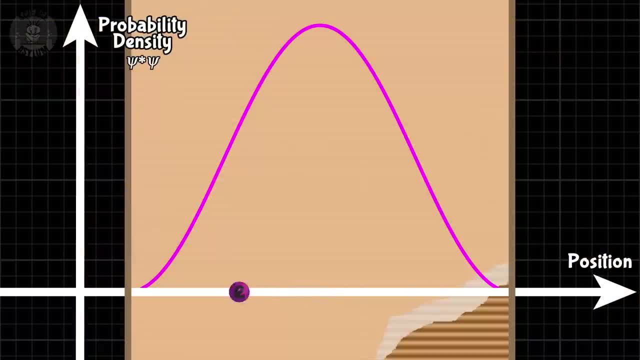 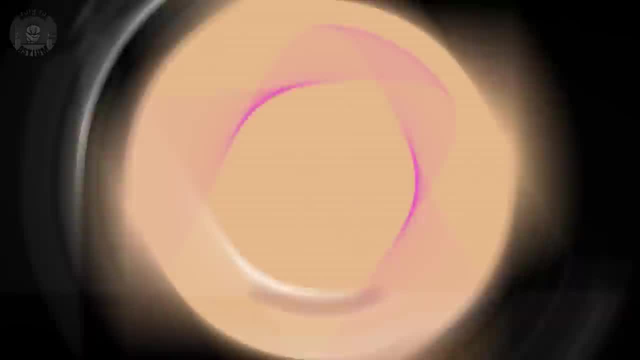 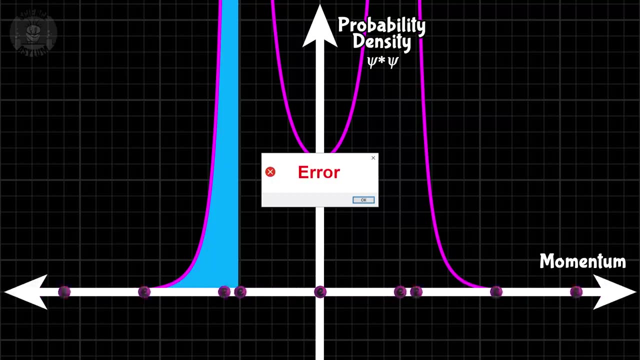 Then you make that thing your input instead. This was in terms of one-dimensional position, so it tells you probabilities in position You want to know about momentum. instead, Just transform the wave function. Any areas you shade now will give you probabilities, As long as the total area is whoa, whoa, wait, whoa, whoa. that wasn't supposed to happen. 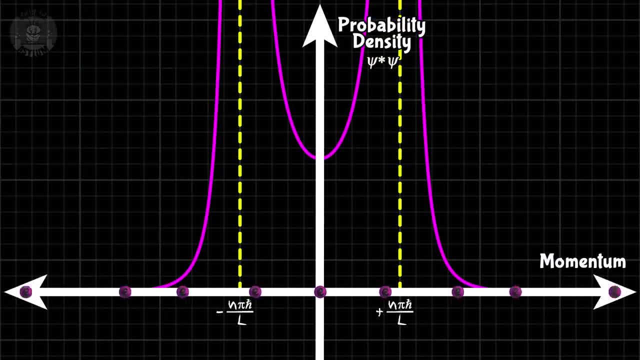 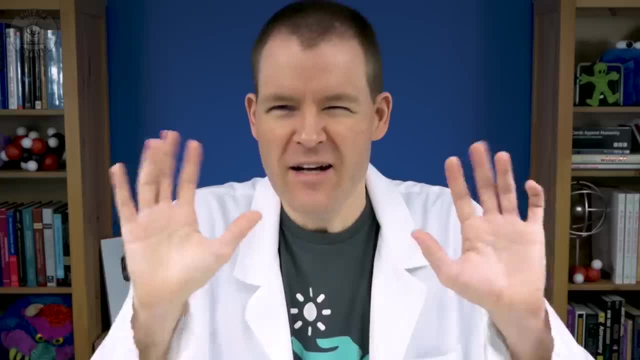 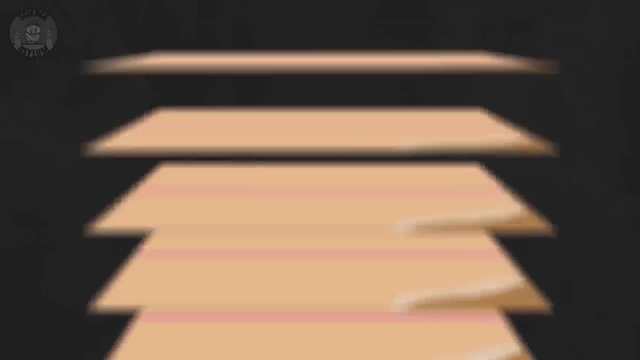 It appears our probability density blows up to infinity in a couple places. What's that mean? Uh, nothing profound. it's just that our example is a bit too simplified. In other words, I was lazy. When you make a particle box that's infinitely deep, infinity is bound to show up in a few results. 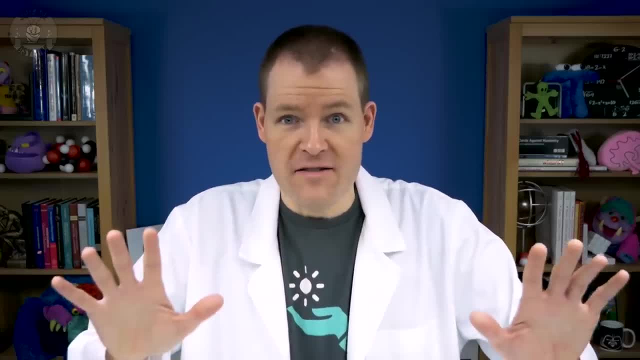 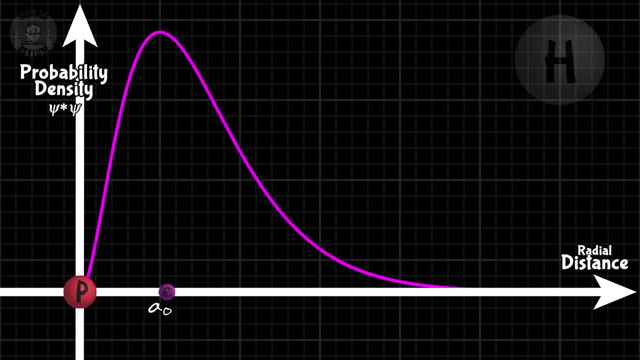 I just happened to find one That doesn't invalidate the whole process, though It works if you choose a model that's a little more realistic. Here's a more accurate probability density for the electron in a hydrogen atom. The input is the distance from the center of the atom. 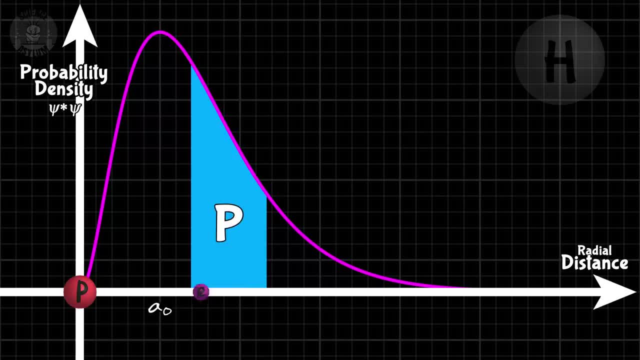 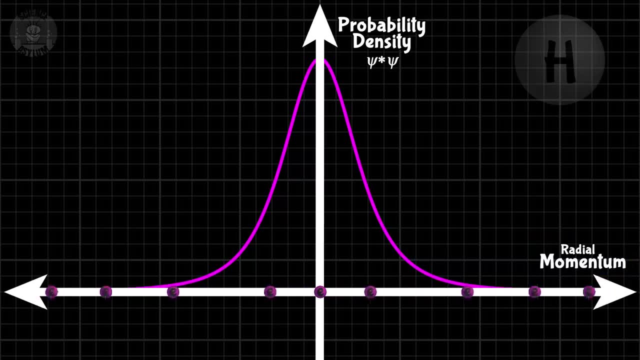 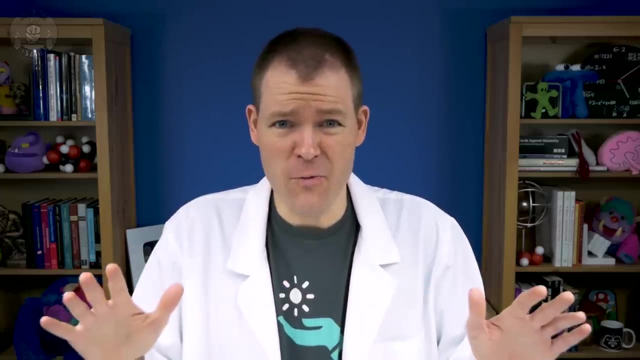 Just like before, any shaded area gives you the probability of finding the electron within that range of distances. If you transform it so that momentum is your input, you can find the probabilities for momentum instead. See no infinities. this time You can write the wave function in terms of anything you want to know. 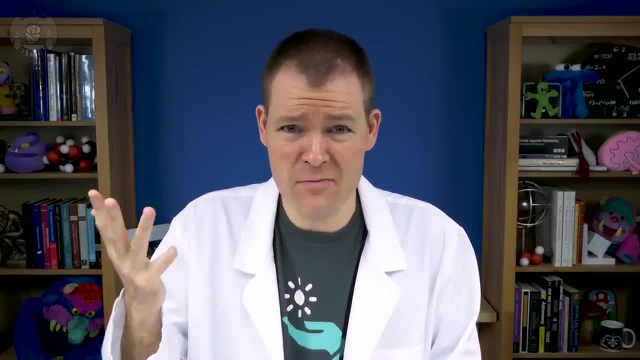 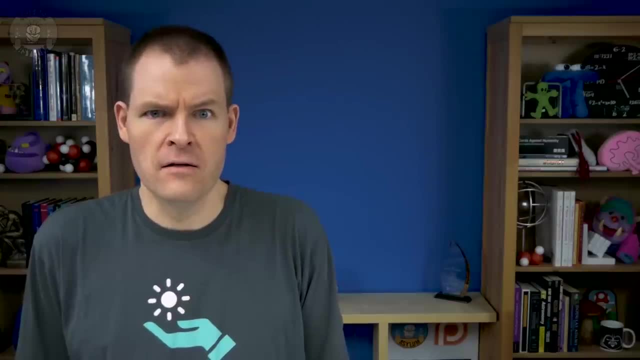 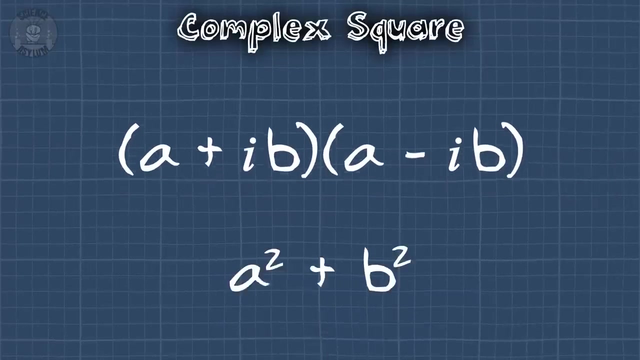 Position, energy, linear momentum, angular momentum, whatever. It's the same wave function, just set up to accept different inputs. So what's a quantum wave function? It's a mathematical entity that has no physical meaning, But if you take its complex square, you give it meaning as a probability density. 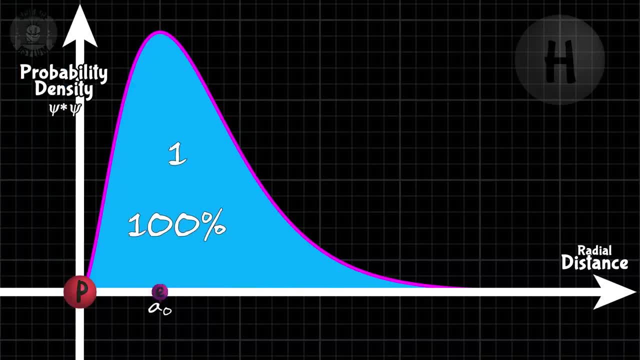 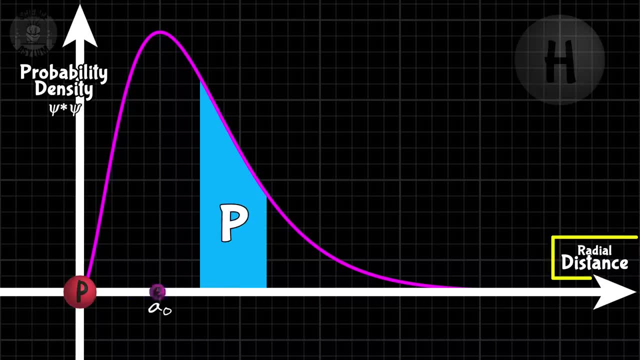 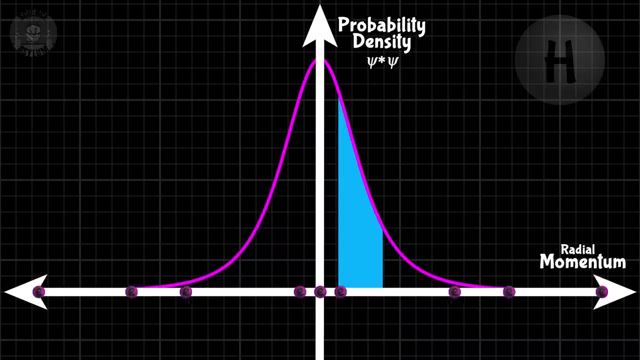 The total area shaded by it should be 1 or 100%, So any smaller area you shade will give you the probability of finding those values when you transform it. If you're interested in another property, you just transform the wave function, But the same rules apply. 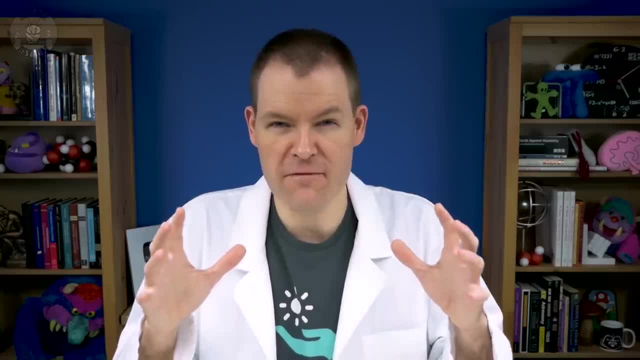 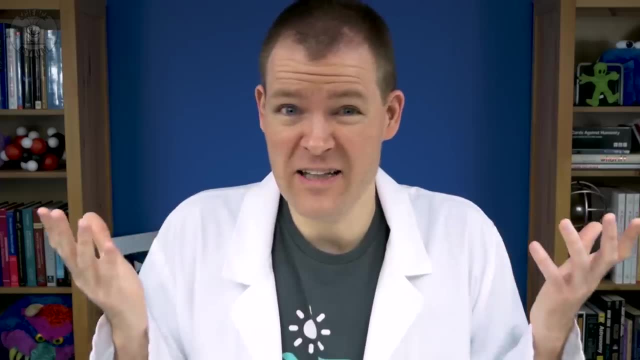 Shaded areas are probabilities. A single quantum wave function contains all the probabilities we might want to know about any property of a quantum particle, And ultimately that's all we get to know. So did this help you understand quantum mechanics a little better? 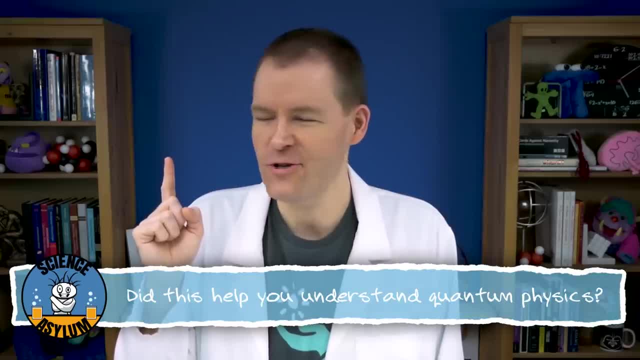 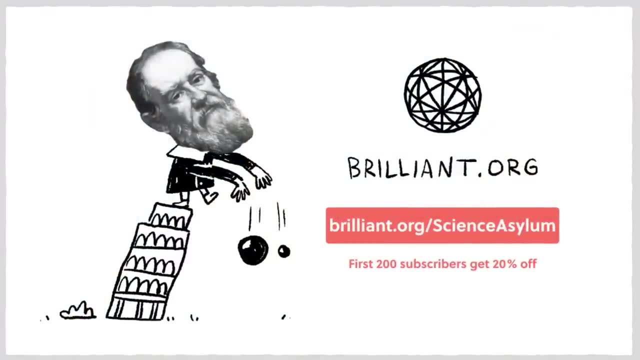 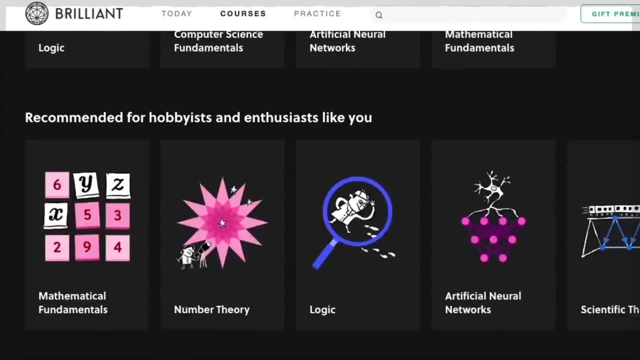 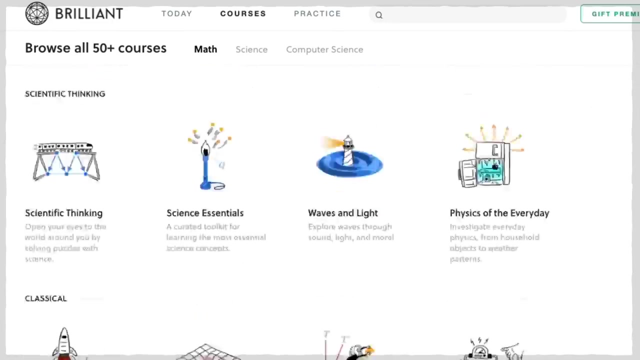 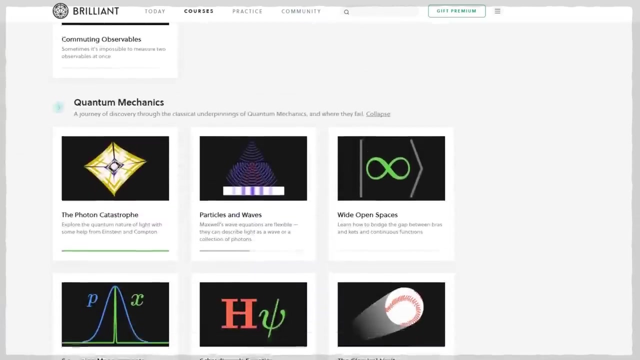 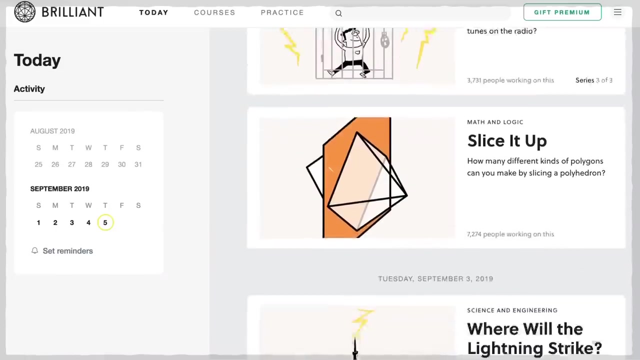 Let us know in the comments. Thanks for liking and sharing this video. Don't forget to subscribe if you'd like to keep up with us. And until next time, remember it's OK to be a little crazy. Brilliant is for ambitious and curious people who want to excel at problem solving and understanding. 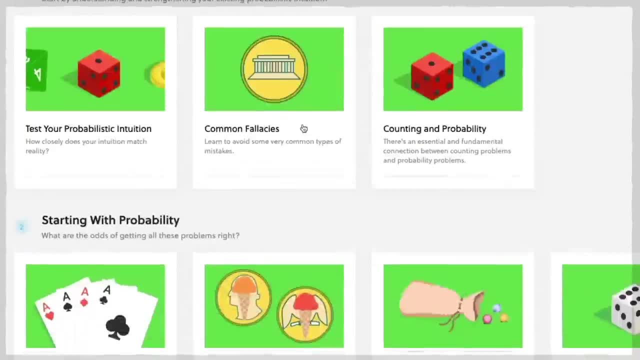 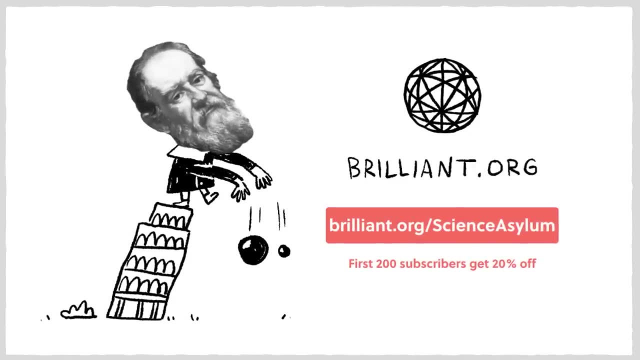 the world. It's a great complement to watching educational videos with well-curated sequences of problems that help you master all sorts of technical subjects. If this sounds like a service you'd like to use, go to Brilliantorg slash Science Asylum today.